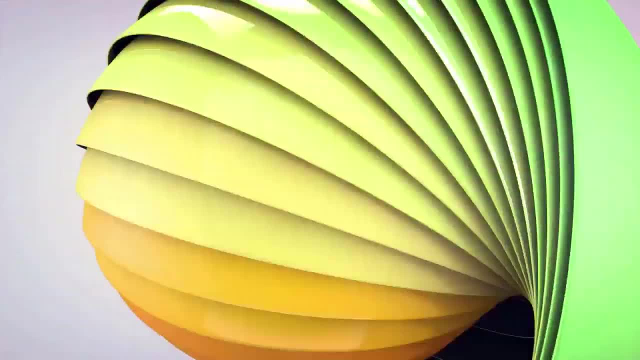 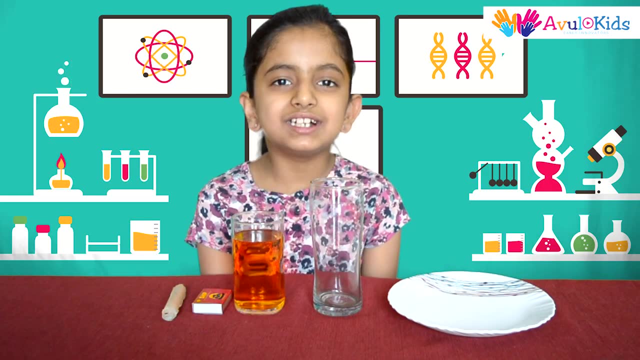 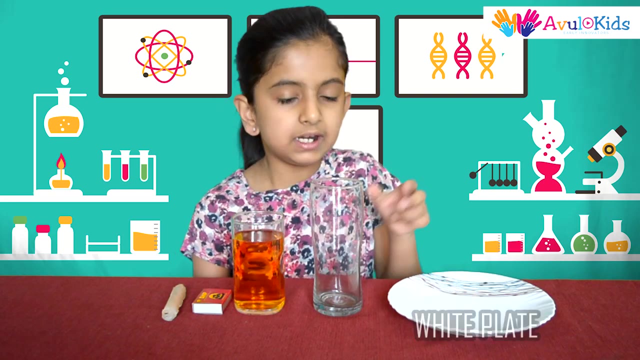 Hi friends, I am Nandini. Welcome to Awful Kids. Today I am going to show you an easy experiment based on vacuum. For this you will need a white plate, an empty glass, some coloured water, matchsticks and a candle. 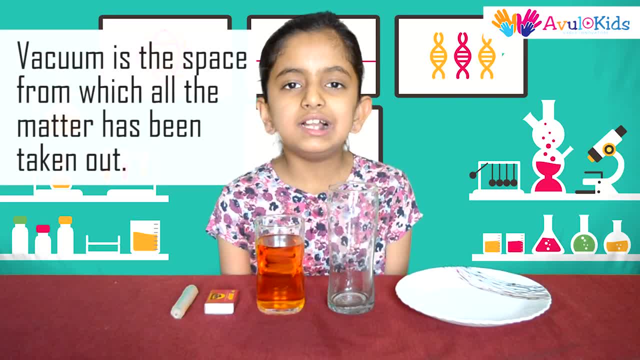 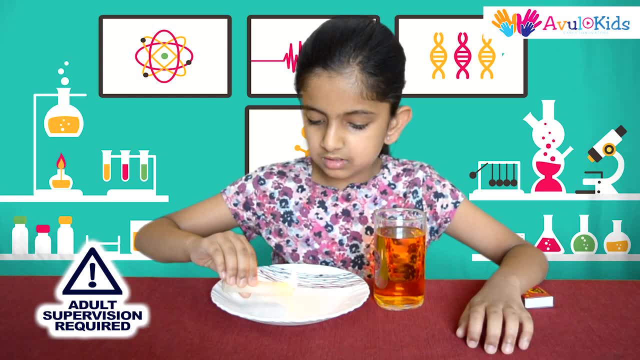 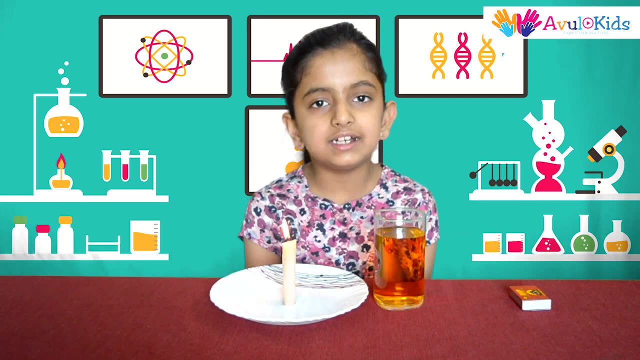 So what is vacuum? Vacuum is the space from which all the matter has been taken out. First light up the candle, Then put a few drops of wax on the plate and then fix the candle, Then wait for few minutes and let it dry. 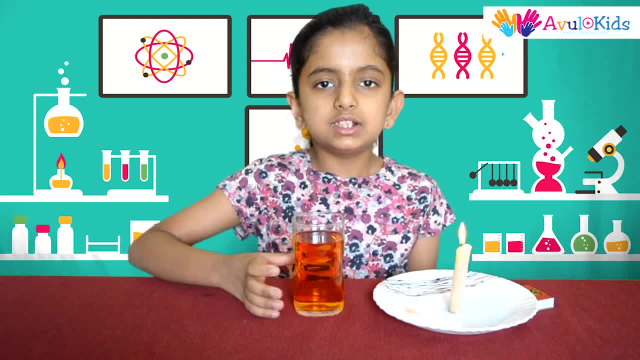 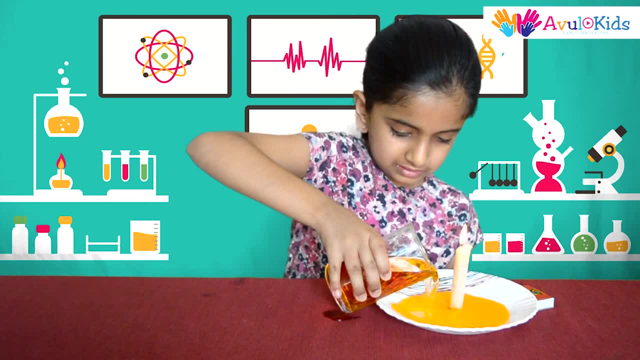 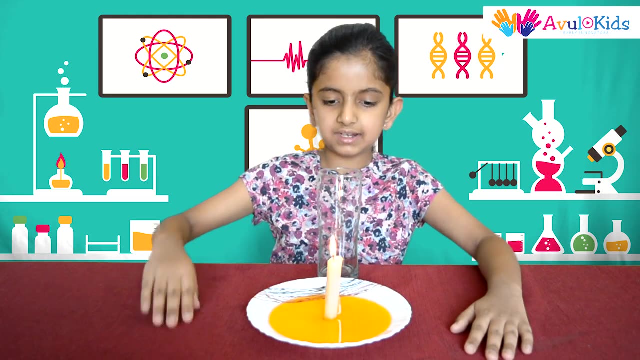 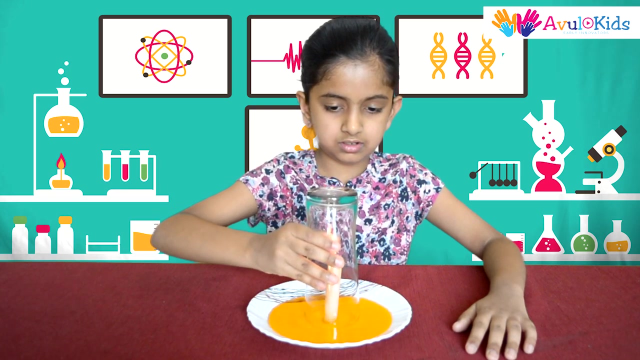 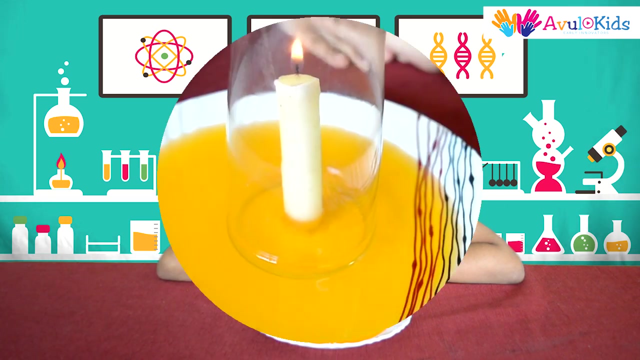 Once the candle is fixed on the plate, then carefully pour some coloured water inside the plate. After pouring water in the plate, carefully cover the candle. Do the same with the empty glass and observe. As you can see, the candle has extinguished. Now let's see how to remove the wax from the plate. 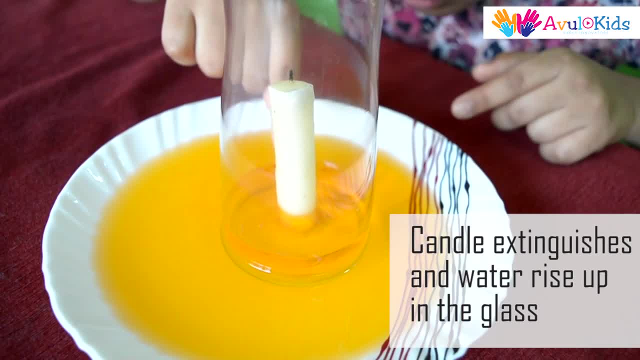 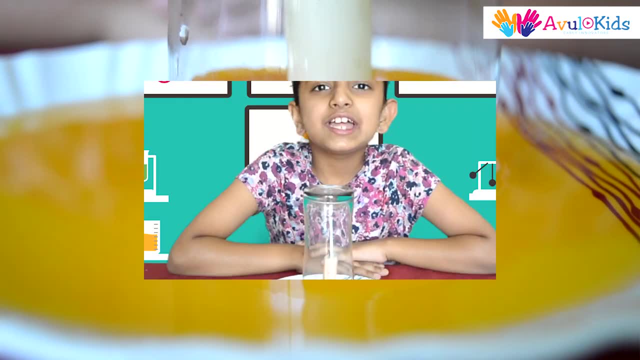 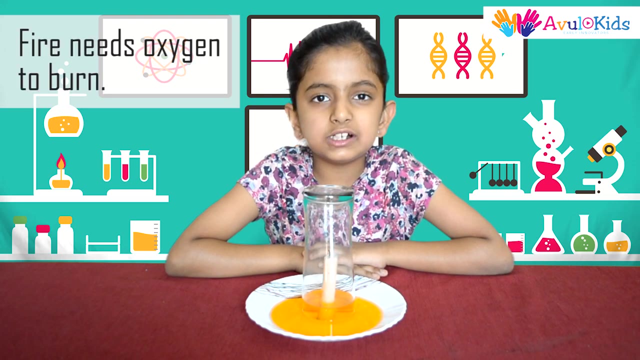 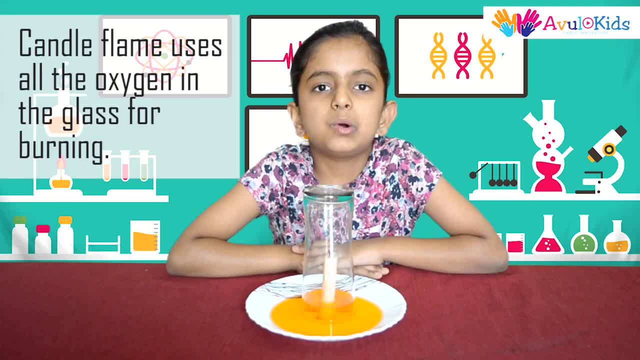 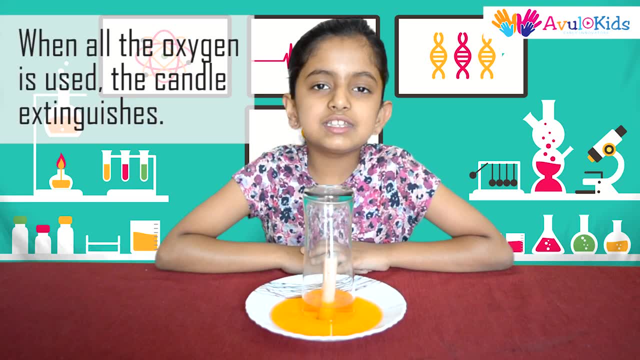 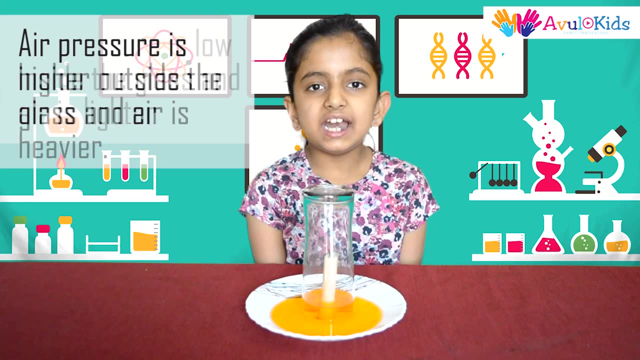 And when we cover the candle with an empty glass, the candle uses up all the oxygen available inside the glass And when the oxygen is all used up, the candle extinguishes itself. Now the air pressure inside the glass is low and the air is lighter, And the air pressure outside the glass is higher and the air is heavier. 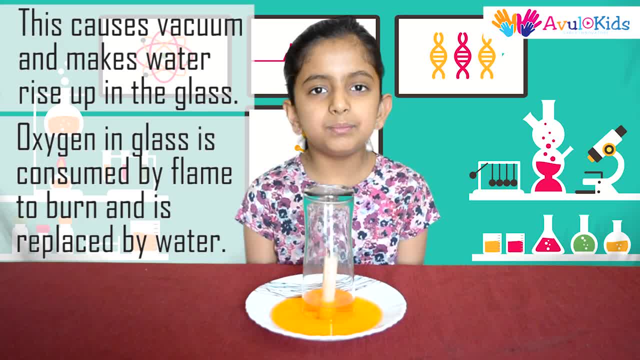 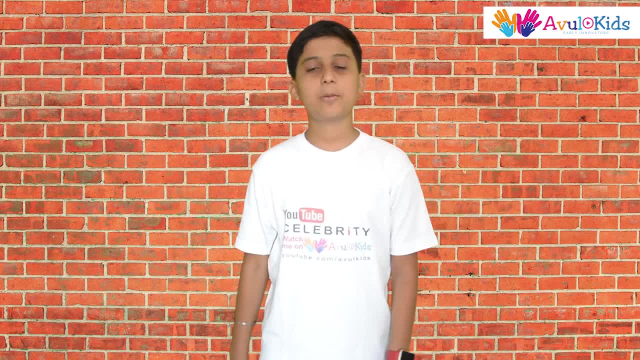 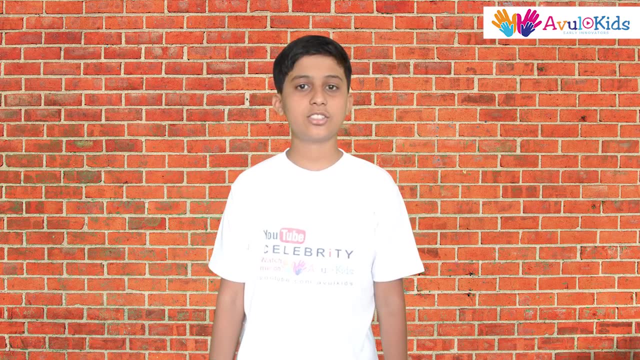 This causes vacuum and makes the water rise up in the glass. Thanks for watching. Hope you enjoyed my video. For more videos, subscribe to our channel. Please keep watching our videos on our channel and don't forget to subscribe to our channel. You can also share your videos with us on our channel.